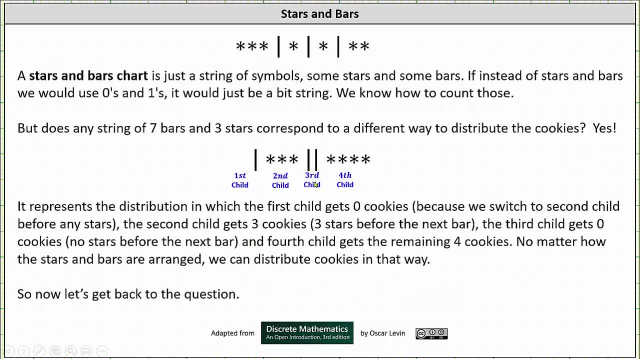 we switch to the third child, but then we switch again to the fourth child, indicating the third child gets zero cookies and the fourth child gets the remaining four cookies. So, no matter how these stars and bars are arranged, we can distribute cookies in that way. So now let's get. 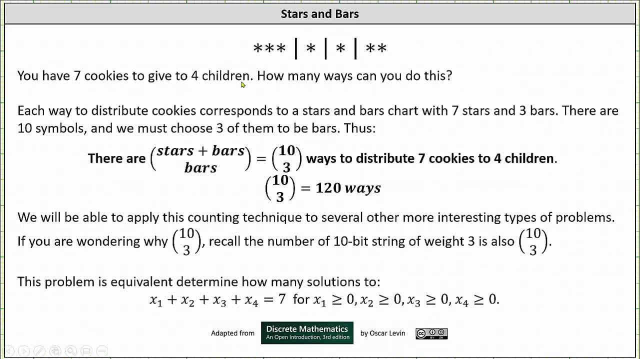 back to our question Again. you have seven cookies to give to four children. How many ways can you do this? Each way to distribute cookies corresponds to a stars and bars chart. with seven stars and three bars. There are a total of ten symbols and we must choose three of them. 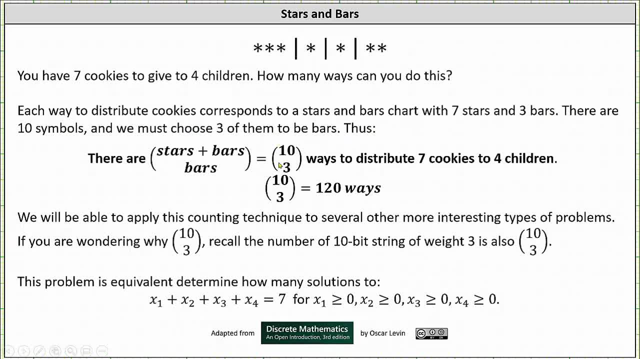 to be bars And therefore there are ten choose three ways to distribute seven cookies to four children, which is 120 ways. Notice how ten choose three is formed by stars plus bars- choose bars. But also remember this is equivalent to stars plus bars. choose stars. We will be able to apply. 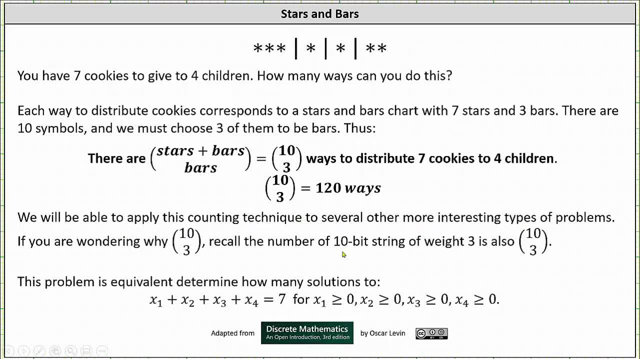 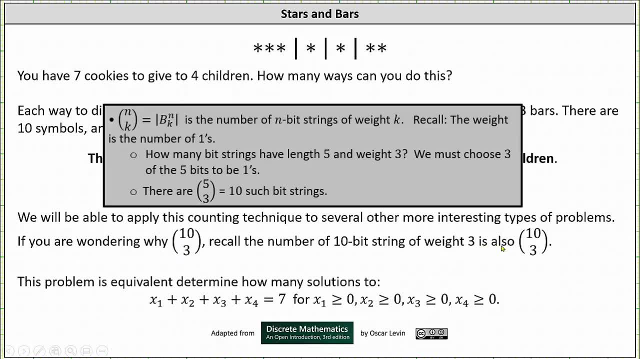 this counting technique to several other interesting types of problems. If you are wondering why ten choose three, recall the number of ten bits, of the number of stars and bars that are in the number of bit strings of weight. three is ten choose three. This cookie problem is also. 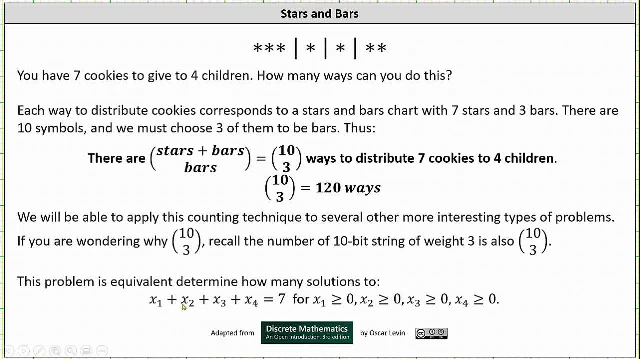 equivalent to the number of solutions to the equation x1 plus x2 plus x3 plus x4 equals seven for x1, x2, x3, x4, all greater than or equal to zero, And this should make sense. Notice: x1, x2, x3, x4. 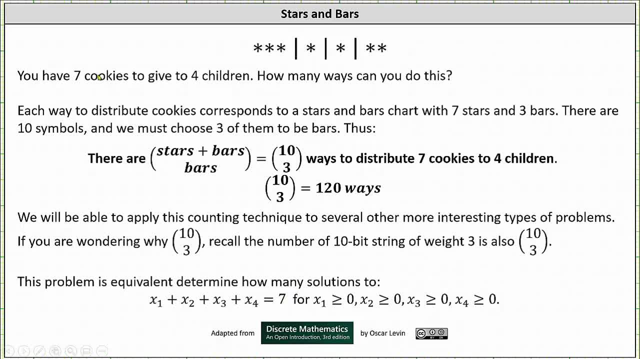 would be the four children and the sum is seven because we have seven cookies. So, looking at the stars and bars chart above, in terms of the equation, this represents the solution where x1 equals three, x2 equals one, x3 equals one and x4 equals two, which does give us a sum of seven and satisfies inequalities. 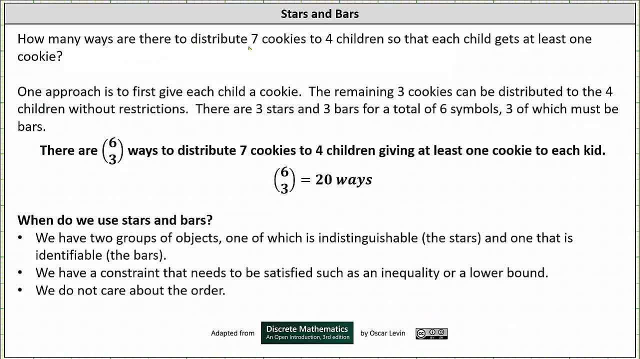 Now let's extend our question. How many ways are there to distribute seven cookies to four children so that each child gets at least one cookie? One approach is to first give each child a cookie. The remaining three cookies can be distributed to the four children without restrictions. There are.